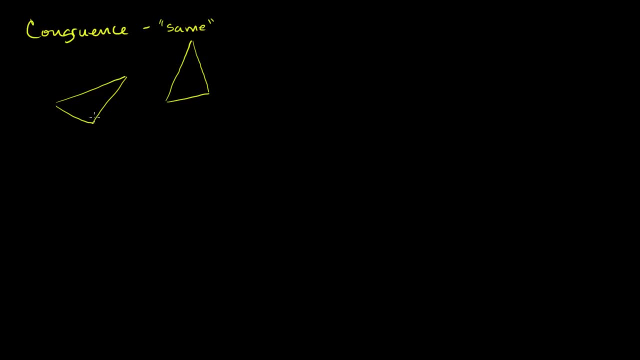 or the angles here. But you can flip it, You can shift it, You can do any and rotate it, So you can shift. Let me write this: You can shift it, You can flip it, You can flip it And you can rotate. 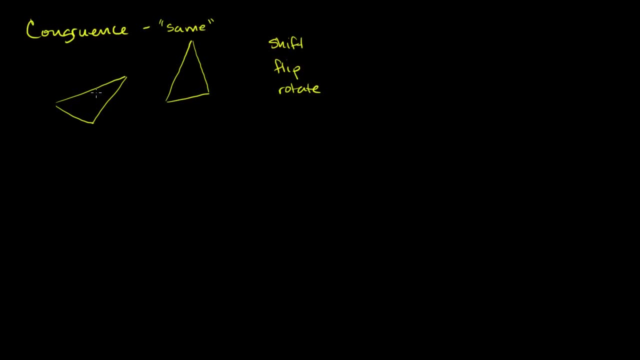 If you can do those three procedures to make the exact same triangle, to make them look exactly the same, then they are congruent. And if you say that a triangle is congruent and let me label these, So let's call this triangle A, B and C. 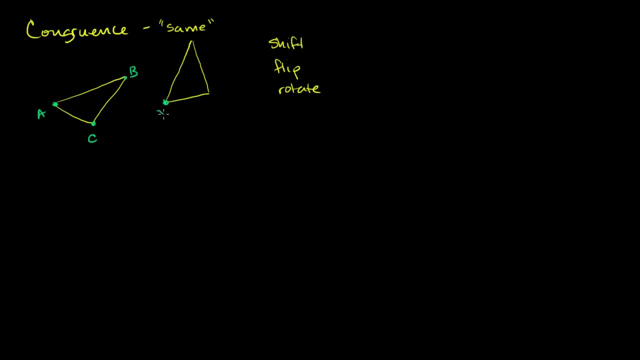 And let's call this D, or let me call it X, Y and Z. So if we were to say, if we make the claim that both of these triangles are congruent, so if we say triangle ABC is congruent and the way you specify it, it looks almost like an equal sign. 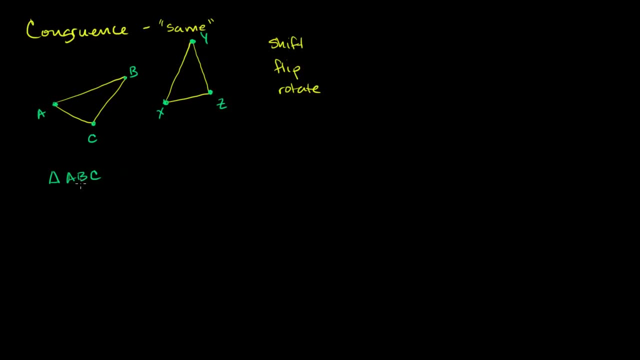 but it's an equal sign with this little curly thing on top. Let me write it a little bit neater. So we would write it like this: If we know that triangle ABC is congruent to triangle XYZ, that means that their corresponding sides, 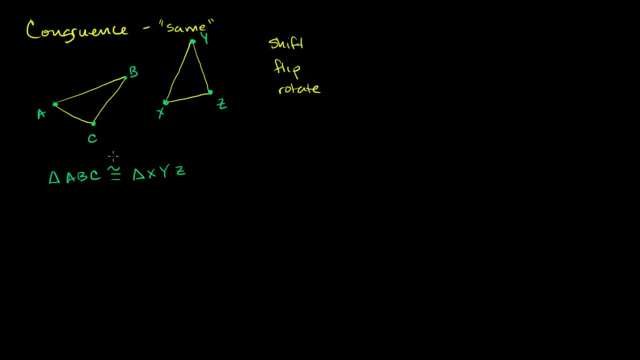 have the same length and their corresponding angles have the same measure. So if we make this assumption, or if someone tells us that this is true, then we know, for example, that AB is going to be equal to XY. The length of segment AB is going. 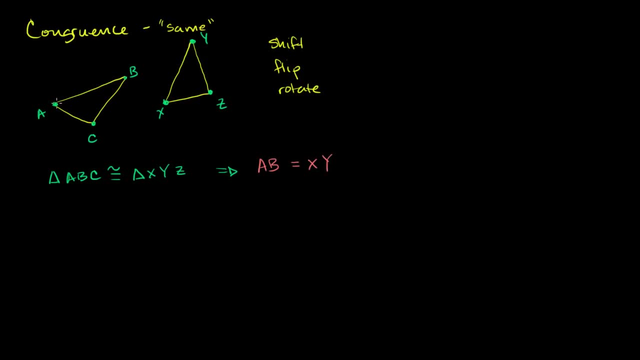 to be equal to the length of segment XY, And we could denote it like this, And I'm assuming that these are the corresponding sides And you can see it: actually, by the way we've defined these triangles, A corresponds to X, B corresponds to Y. 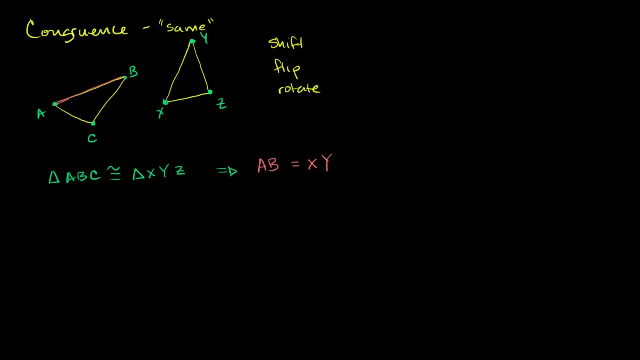 and then C corresponds to Z, Right Right over there. So AB side AB is going to have the same length as side XY, And you can sometimes, if you don't have the colors, you would denote it just like that. 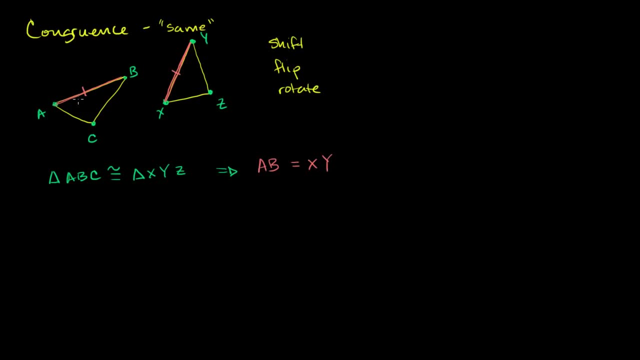 These two lengths are, or these two line segments have the same length, And you can actually say this- and you don't always see it written this way- You could also make the statement that line segment AB is congruent to line segment XY. 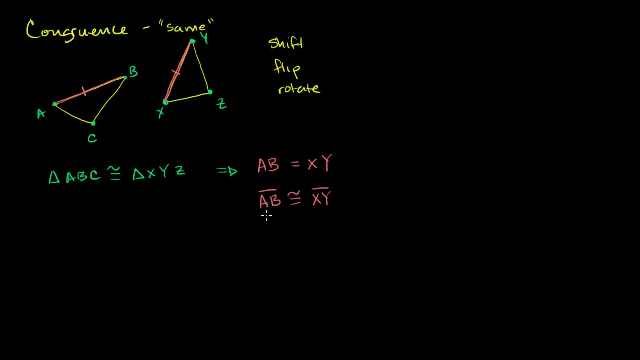 But congruence of line segments, It really just means that their lengths are equivalent. So these two things mean the same thing. If one line segment is congruent to another line segment, that just means the measure of one line segment is equal to the measure of the other line segment. 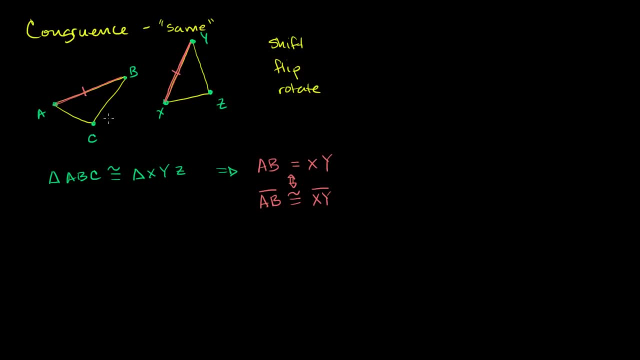 And so we can go through all the corresponding sides If these two characters are congruent. we also know that BC is going to be the length of YZ, assuming that those are the corresponding sides, And we could put that in. Put these double hash marks right over here. 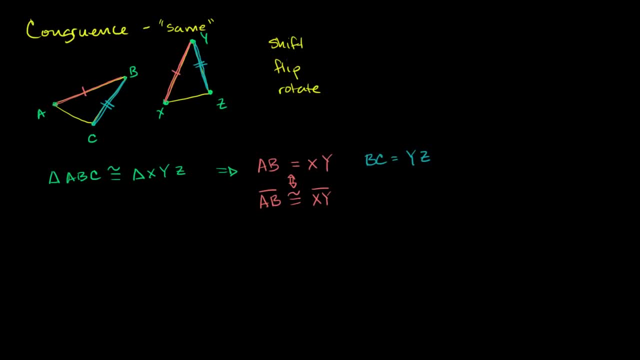 to show that these two lengths are the same. And then, if we go to the third side, we also know that these are going to have the same length, or the line segments themselves are going to be congruent. So we also know that the length of AC. 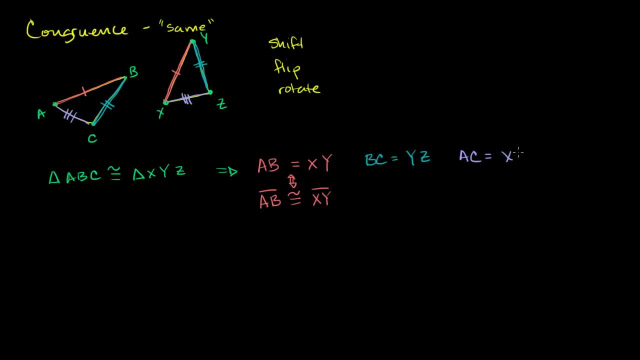 is going to be equal to the length of XZ. Not only do we know that all of the corresponding sides are going to have the same length. if someone tells us that a triangle is congruent, we also know that all the corresponding angles are going to have the same measure. 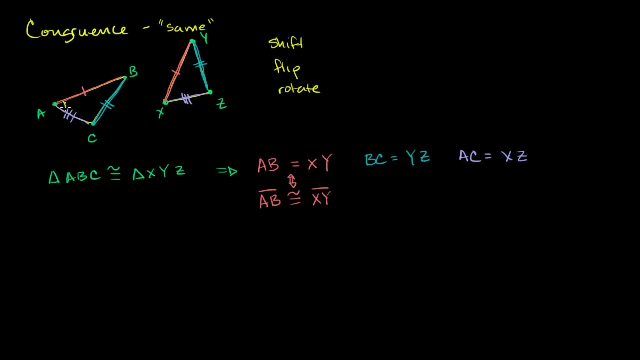 So, for example, we also know that this angle's measure is going to be the same as the corresponding angle's measure, And the corresponding angle is right over here. It's between this orange side and this blue side, or this orange side and this purple side. I should say. 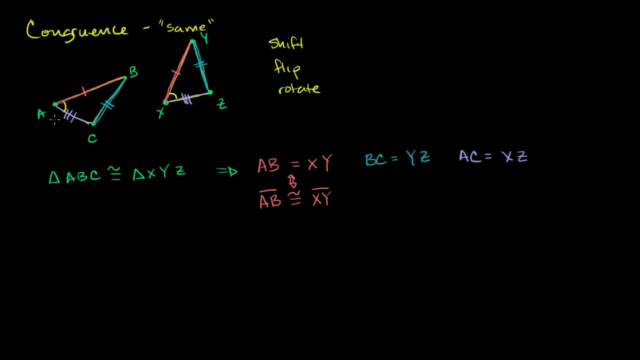 And between the orange side and this purple side. And so it also tells us that the measure of angle is this: BAC. The measure of angle. BAC is equal to the measure of angle of angle. YXZ Measure of angle. let me write that angle symbol a little less. 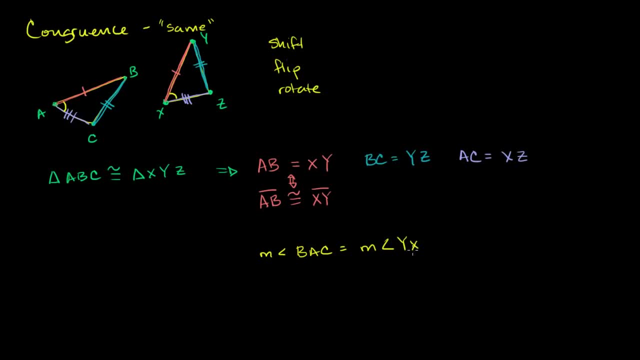 Measure of angle YXZ, YXZ. We could also write that as angle BAC is congruent to angle YXZ. And once again, like line segments, if one line segment is congruent to another line segment, it just means that they're linked. 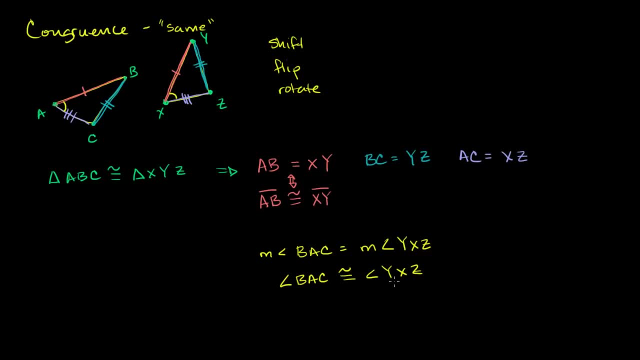 Lengths are equal, And if one angle is congruent to another angle, it just means that their measures are equal. So we know that those two corresponding angles have the same measure. They're congruent. We also know that these two corresponding angles 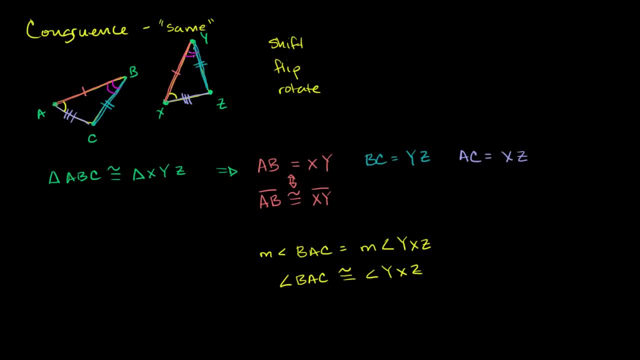 have the same measure, And I'll use a double arc to specify that this has the same measure as that. So we also know that the measure of angle ABC is equal to the measure of angle XYZ. And then, finally, we know that this angle 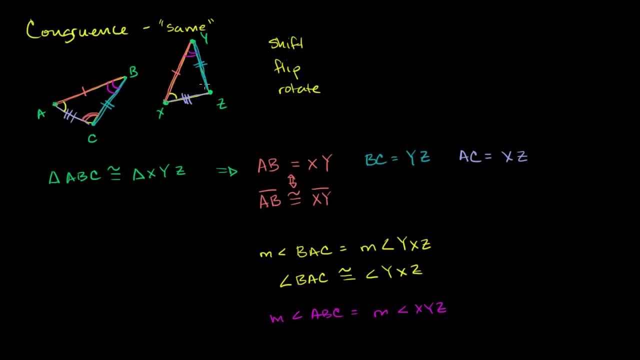 if we know that these two characters are congruent, that this angle is going to have the same measure as this angle, as its corresponding angle. So we know that the measure of angle ACB is going to be equal to the measure of angle XZY. 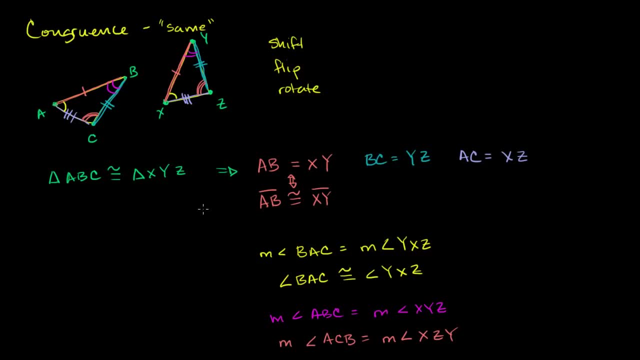 Now, what we're going to concern ourselves a lot with is: how do we prove this? How do we prove congruence? Because it's cool, Because if you can prove congruence of two triangles and all of a sudden, you can make all of these assumptions. 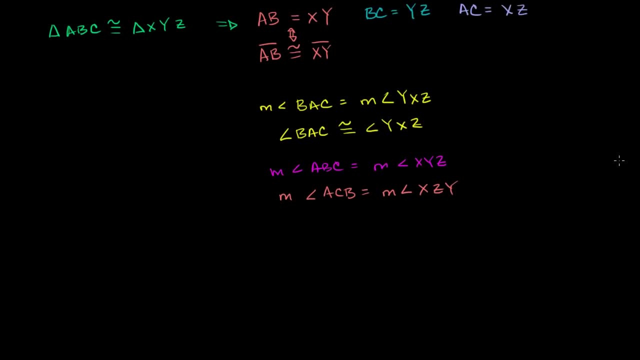 And what we're going to find out, and this is going to be what we could. we're going to assume it, for the sake of kind of an introductory geometry course, that this is an axiom or a postulate or just something that you assume. 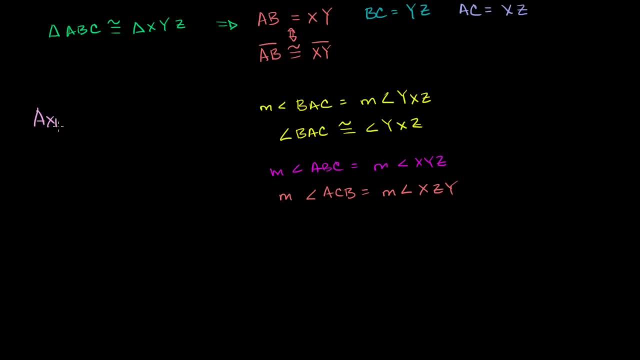 And let me actually just write this down. So an axiom- a very fancy word, Postulate also a very fancy word. It really just means things that we're going to assume are true. An axiom is: sometimes there's a little bit of distinction. 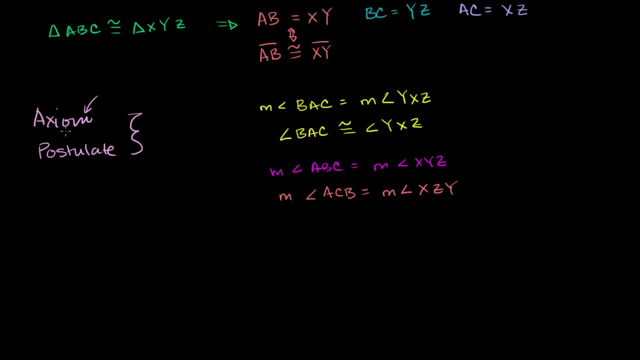 sometimes where someone will say an axiom is something that's self-evident or it seems like a universal truth. that is definitely true and we just take it for granted. You can't prove an axiom. A postulate kind of has that same role. 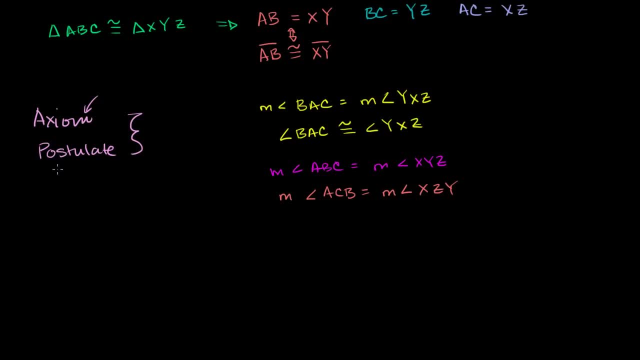 But sometimes you can say: well, let's just assume this is true and see, if we assume that that's true, what we can derive from it, What we can prove if we assume it's true, But for the sake of an introductory geometry class. 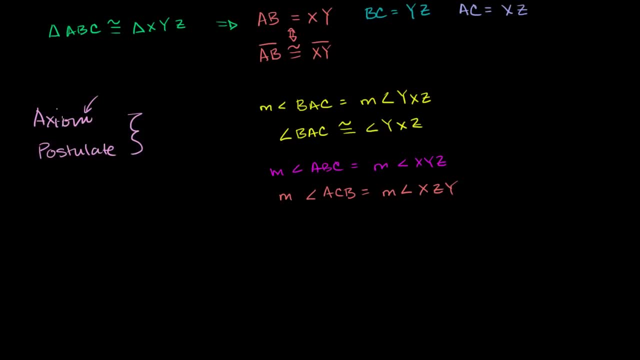 and really in most of mathematics today these two words are used interchangeably: An axiom or a postulate, just very fancy words for things that we take as a given, things that we just will assume. We won't prove them. We will start with these assumptions. 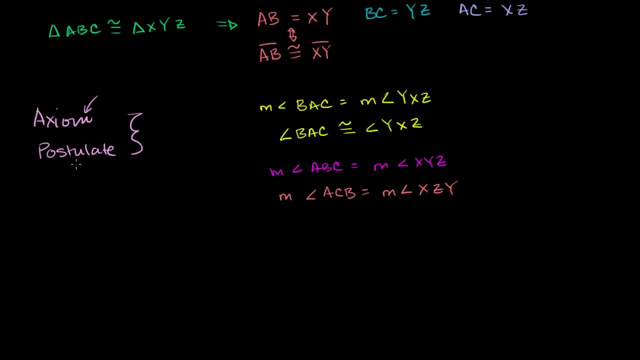 and then we're just going to build up from there, And one of the core ones that we'll see in geometry is the axiom or the postulate that if all of the sides are congruent, or if the lengths of all the sides of the triangle 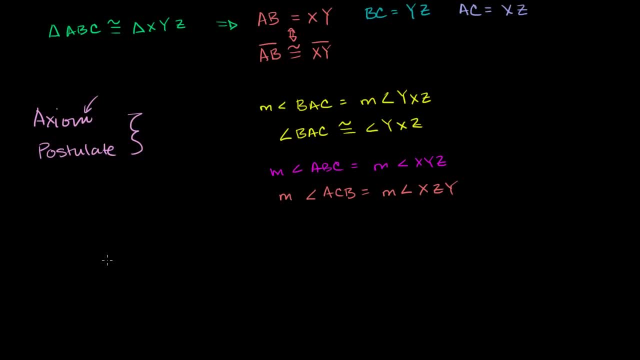 are congruent, then we are dealing with congruent triangles. So it's sometimes called the side side side postulate or axiom. We're not going to prove it here, We're just going to take it as a given. So this literally stands for side side side. 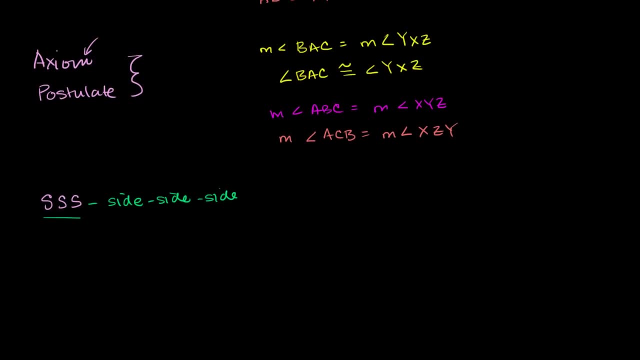 And what it tells us is: if we have two triangles and so let's say that's another triangle right over there And we know that corresponding sides are equal, So we know that this side right over here is equal in length to that side. 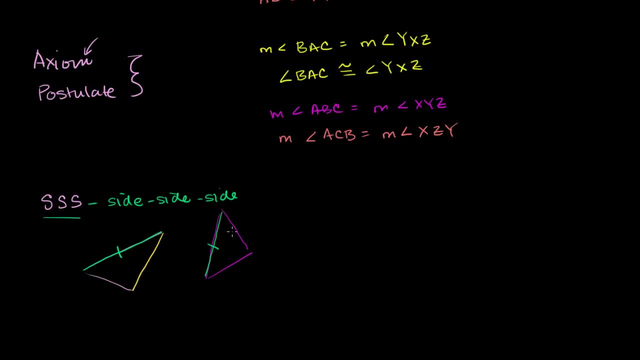 We know that this side right over here is equal in length to that side right over there, And we know that this side over here is equal in length to this side over here, Then we know, and we're just going to take this as an assumption and we can build up off of this, 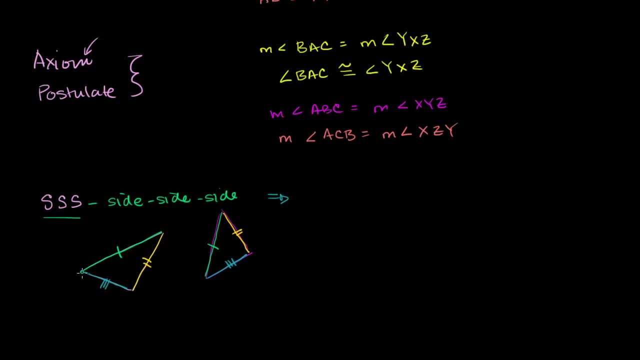 We know that they are congruent, that these two triangles are congruent to each other. I didn't put any labels there so it's kind of hard for me to refer to them, But these two are congruent triangles And what's powerful there is if we 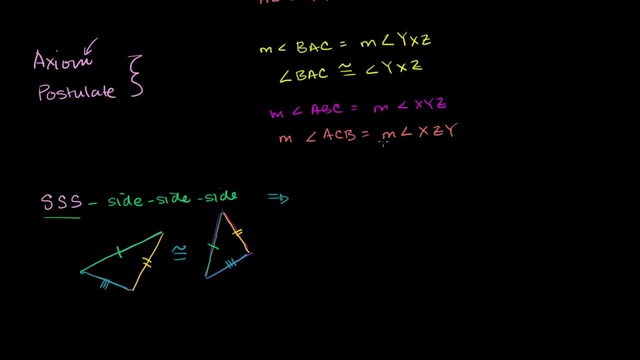 know all of the corresponding sides are equal, then we know they're congruent And then we can make all of the other assumptions, which means that the corresponding angles are also equal, so that we know that that's going to be congruent to that, or have the same measure. 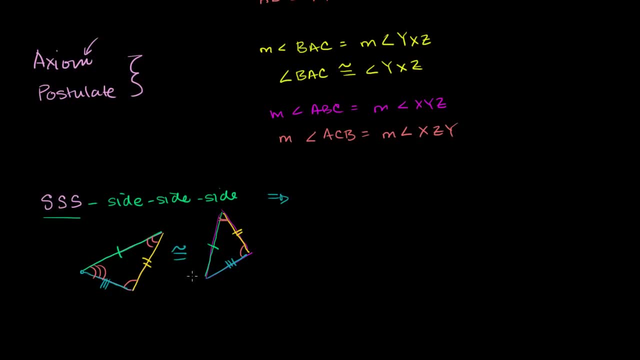 That's going to have the same measure as that, And then that is going to have the same measure as that, right over there. And to see why that is a reasonable axiom or a reasonable assumption or a reasonable postulate to start off with, let's start with one triangle. 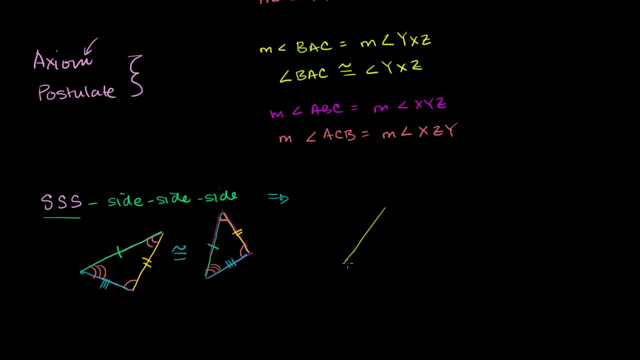 So let's say I have this triangle right over here, So it has that side, and then it has that side, and then it has that side right over here, And what I'm going to do is see if I have another triangle that has the exact same side lengths. 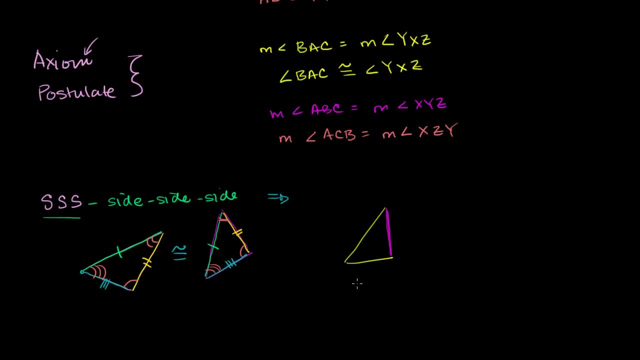 is there any way for me to construct a triangle with the same side lengths that is different, that can't be translated to this triangle through flipping, shifting or rotating. So we assume that We assume this other triangle is going to have a side that's the same length as that one right? 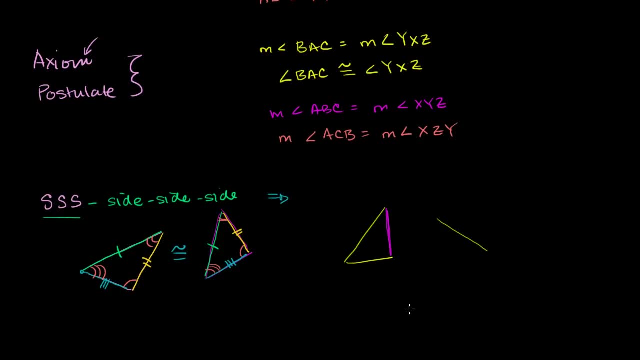 over there. So I'll try to draw it like that, roughly the same length. We know it's going to have a side. that's that length, So it's going to have a side. that's that length. Let me put it on this side just to make it look. 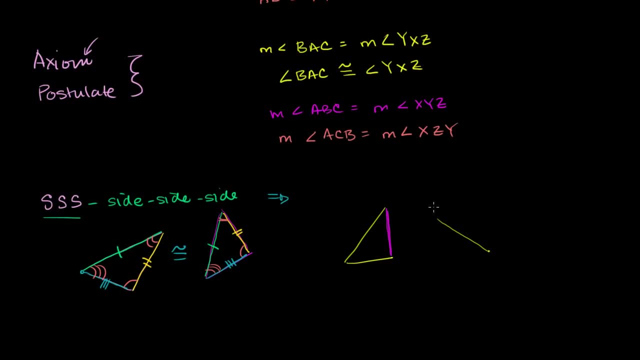 a little bit more interesting. So we know it's going to have a side like that. So I'm going to draw it roughly the same length, but I'm going to try to do it at a different angle, And we know it's going to have a side that looks like that. 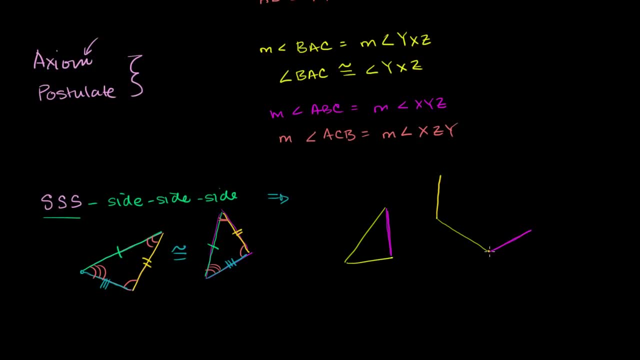 And so let me I'll put it right over here. It's about that length right over there, And so clearly this isn't a triangle. In order to make it a triangle, I'll have to connect this point to that point right over there. 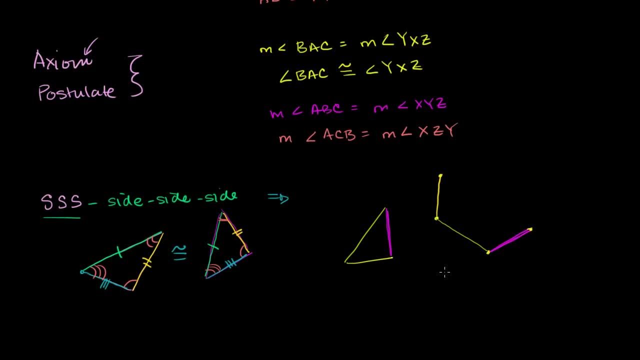 And really there's only two ways to do it. I can rotate it around that little hinge right over there. If I connect them over here, then I'm going to get a triangle that looks like this, which is really just a flipped. 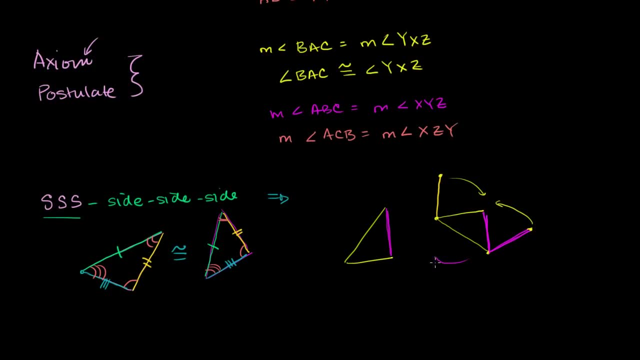 Am I visualizing it right? Yeah, just a flipped version. You could rotate it a little bit back this way, but then you'd have the magenta on this side and the yellow on this side, And then you could flip it vertically. 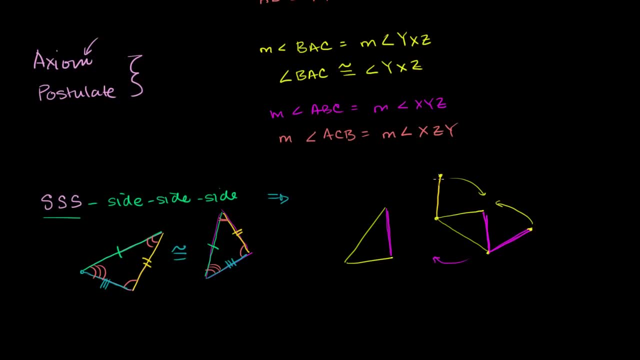 and then it would look exactly like this. Our other option to make these two points connect is to rotate them out this way, And then the yellow side is going to be here, And then the magenta side is going to be right over here. 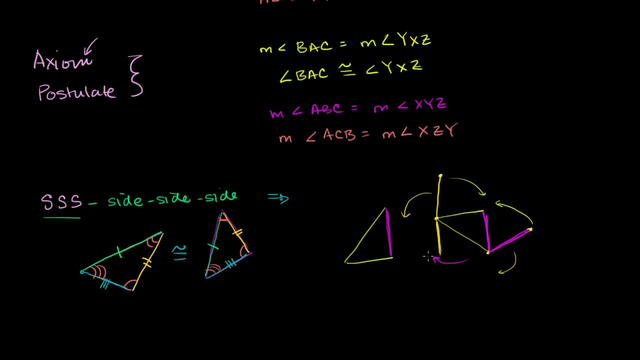 And that's not magenta, The magenta side. It's going to be just like that, And if we do that, then we actually just have to rotate it. We just have to rotate it around to get that exact triangle. So this isn't a proof. 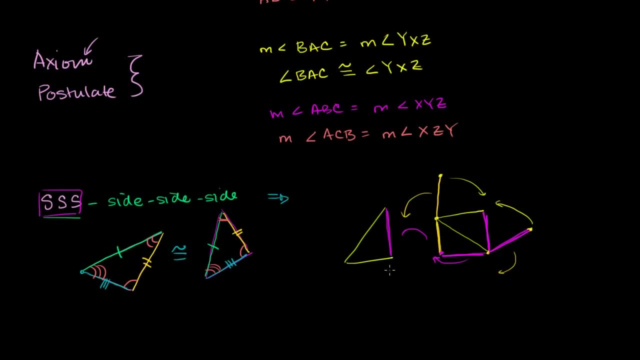 And actually we're just going to start assuming that this is an axiom, But hopefully you see that it's a pretty reasonable starting point that if all of the sides, all of the corresponding sides of two different triangles are equal, then we know that they are congruent. 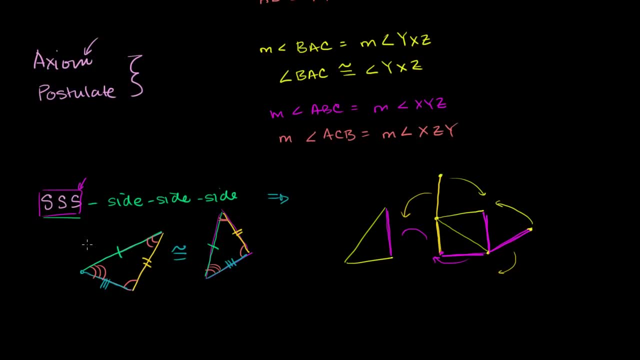 We're just going to assume it is an axiom that we're going to build off of, that they are congruent, And then we also know that all of the corresponding angles are going to be equivalent.